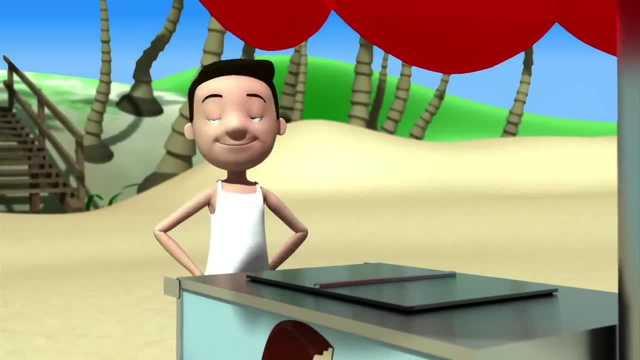 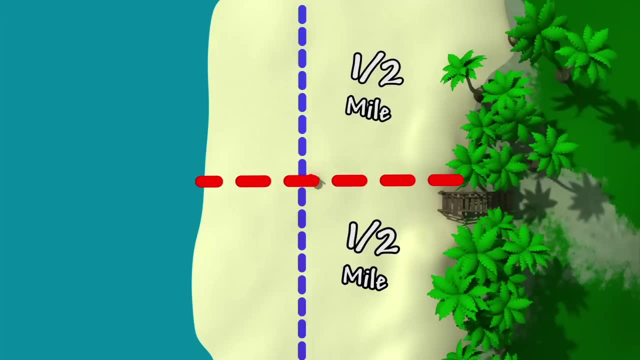 and you have no competition. Where would you place your cart in order to sell the most product? In the middle. The one half mile walk may be too far for some people at each end of the beach, but your cart serves as many people as possible. One day you show. 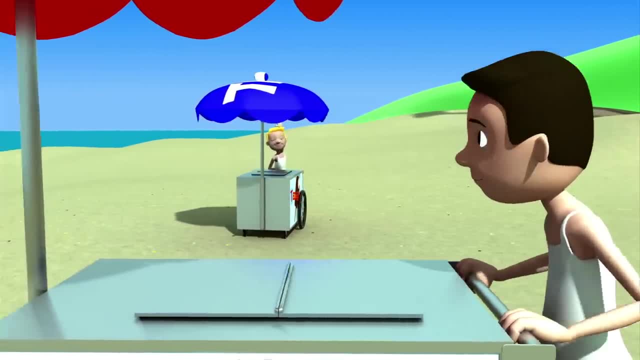 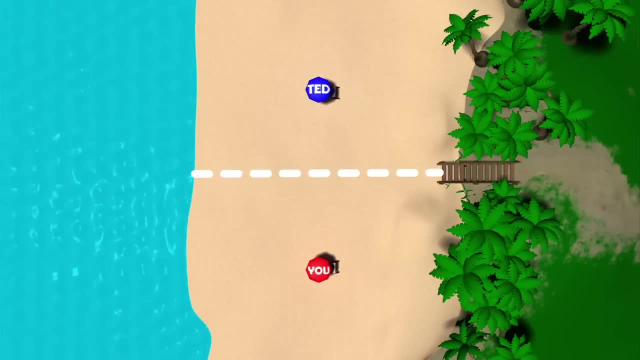 up at work just as your cousin, Teddy, is arriving at the beach with his own ice cream cart. In fact, he's selling exactly the same type of ice cream as you are. You agree that you will split the beach in half In order to ensure that customers don't have to walk too far? 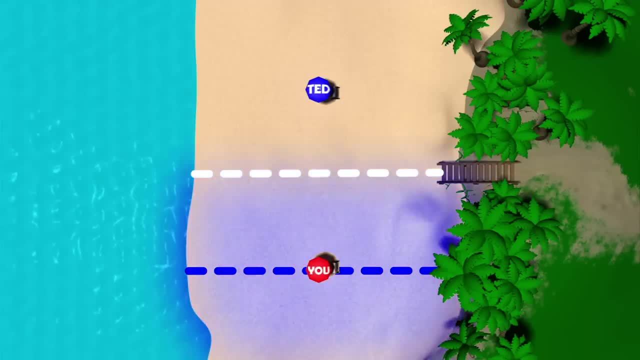 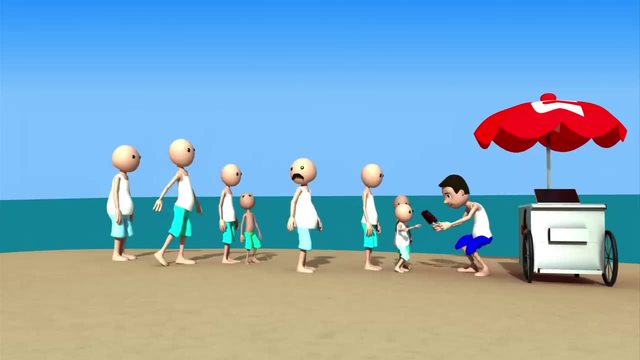 you set up your cart a quarter mile south of the beach center, right in the middle of your territory. Teddy sets up a quarter mile north of the center in the middle of Teddy territory. With this agreement, everyone south of you buys ice cream from you. 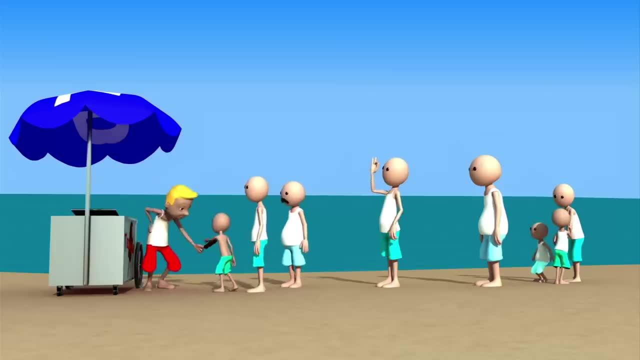 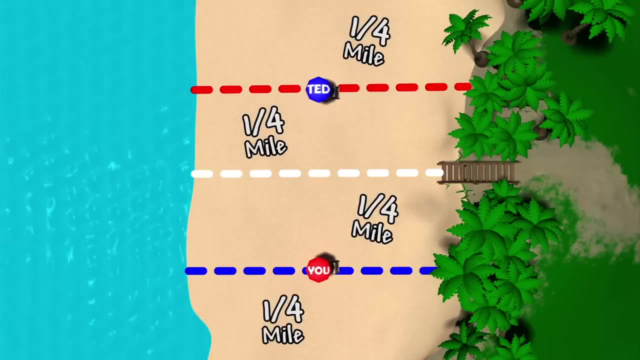 Everyone north of Teddy buys from him, and the 50% of beach goers in between walk to the closest cart. No one walks more than a quarter of a mile and both vendors sell to half of the beach goers. Game theorists consider this a socially optimal solution. It minimizes. 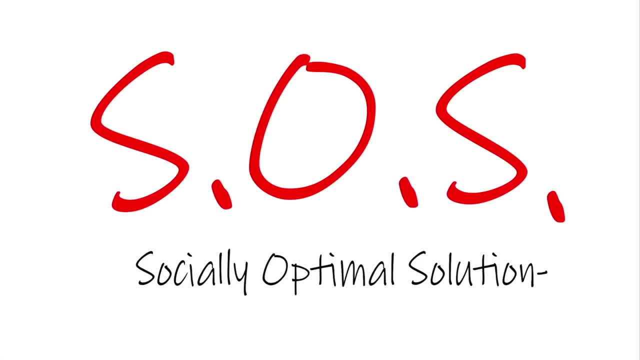 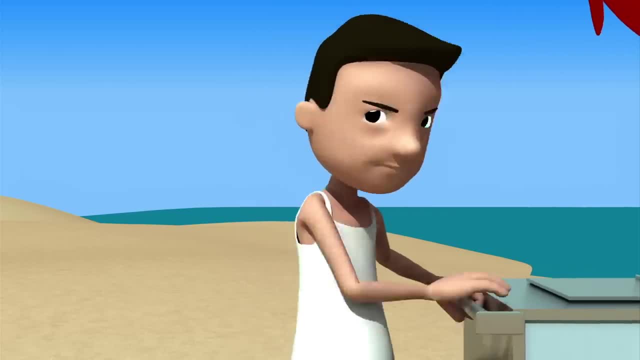 the maximum number of steps any visitor must take in order to reach an ice cream cart. The next day. when you arrive at work, Teddy has set up his cart in the middle of the beach. You return to your location a quarter mile south of center and get the 25% of customers. 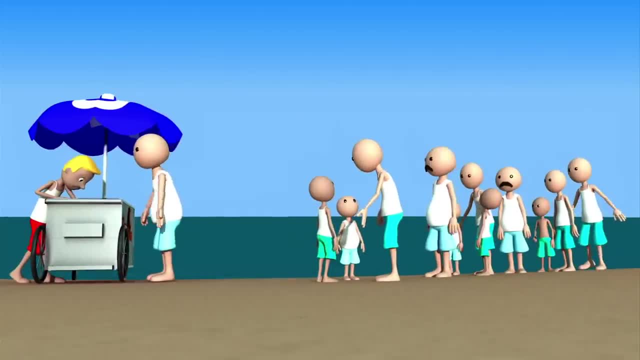 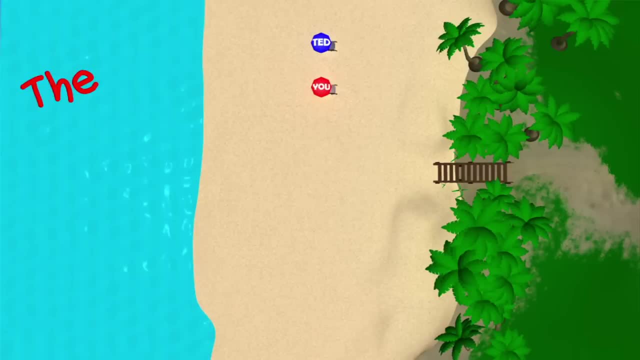 to the south of you. Teddy still gets all of the customers north in Teddy territory, but now you split the 25% of people in between the two carts. Day three of the ice cream wars. you get to the beach early and set up right in the center of Teddy territory. 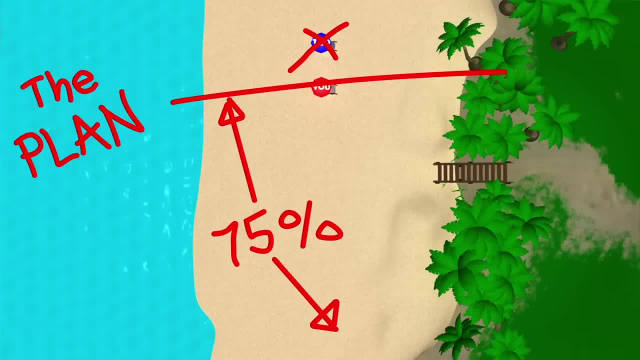 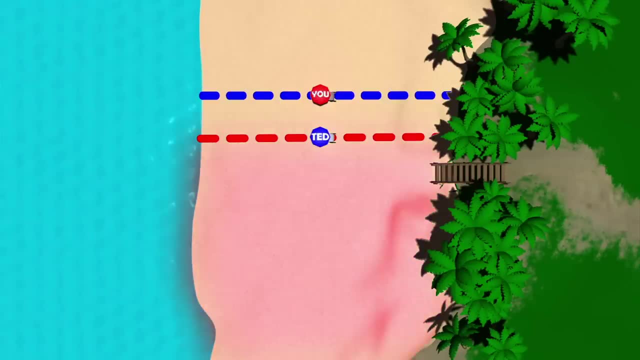 assuming you'll serve the 75% of beach goers to your south, leaving your cousin to sell to the 25% of customers to the north. When Teddy arrives, he sets up just south of you, stealing all of the southerly customers and leaving you with a small group of people to 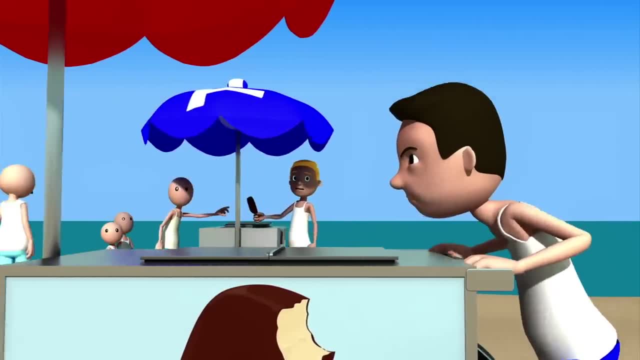 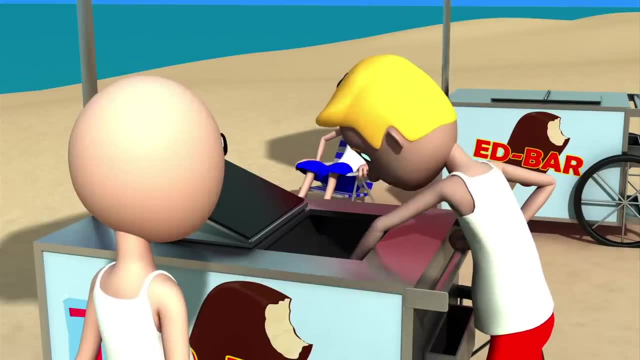 the north. When you're done, you move 10 paces south of Teddy to regain your customers. When you take a midday break, Teddy shuffles 10 paces south of you and again steals back all the customers to the far end of the beach. Throughout the course of the day, both of you continue. 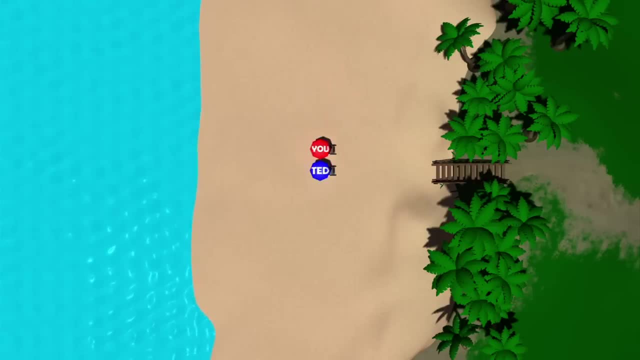 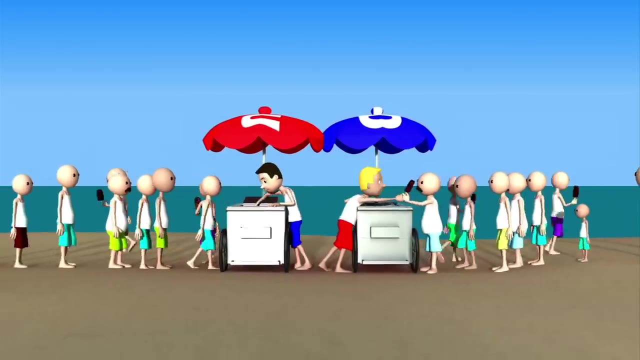 to periodically move south towards the bulk of the ice cream buyers until both of you eventually end up at the center of the beach, back to back, each serving 50% of the ice cream hungry beach goers. At this point, you and your competitive cousin have reached what game theorists call a Nash.